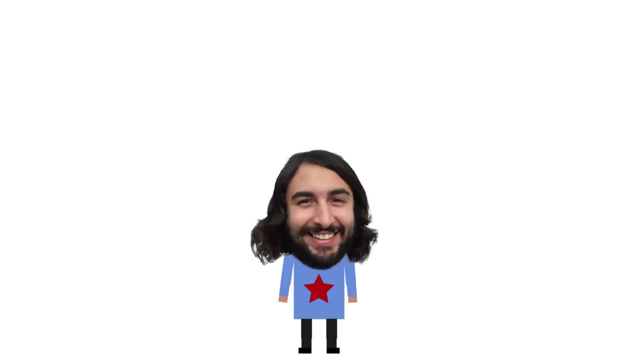 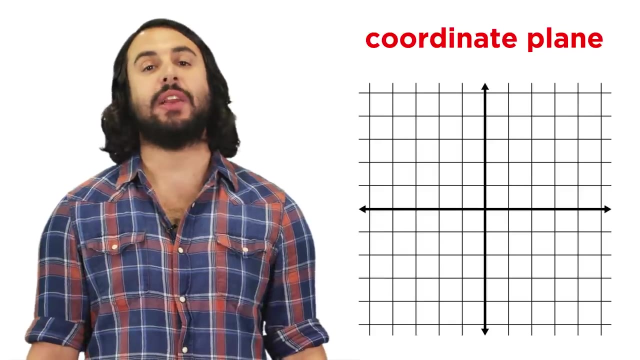 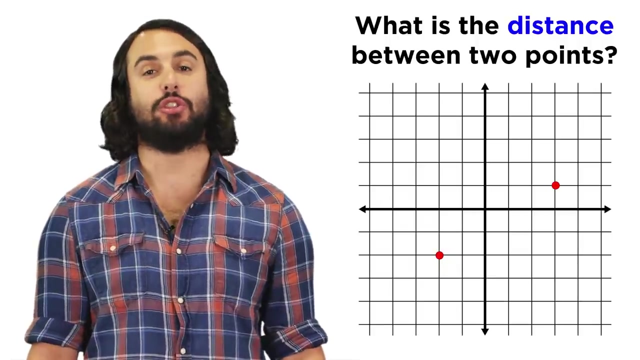 It's Professor Dave. let's learn the distance formula As we navigate the coordinate plane in our algebraic adventures. one thing we might want to do is find the distance between two points. Luckily, we are well equipped to do this, since we know the Pythagorean theorem. 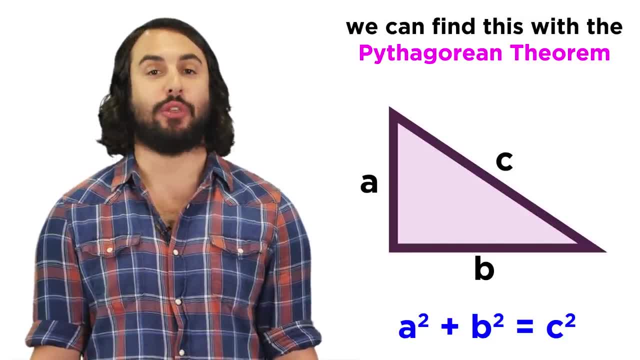 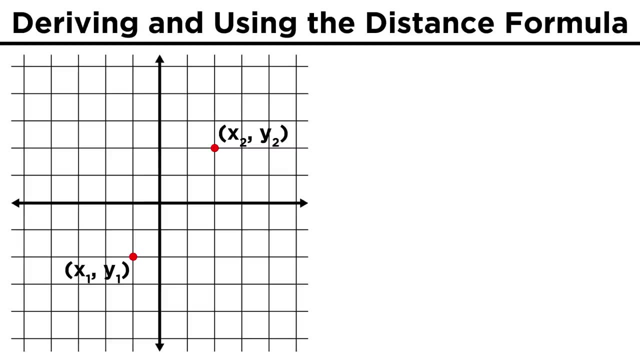 If you need to review it, check out the tutorials on how to use the theorem, as well as how the theorem was derived in the geometry portion of this playlist. Otherwise, let's just select two points in the coordinate plane and draw a line between them. 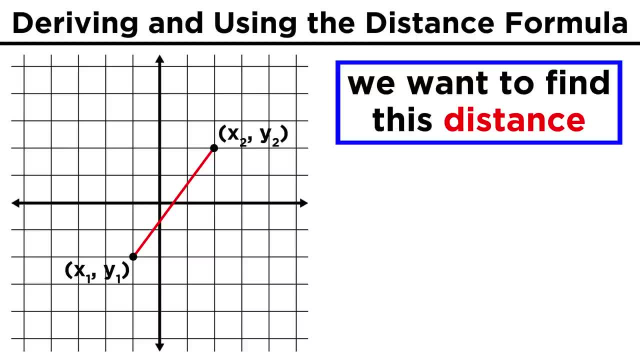 The length of this line is what we are trying to figure out and, in order to get it, we can make a right triangle. This line will be the hypotenuse and the legs will be the horizontal and vertical line segments we need to construct the triangle. 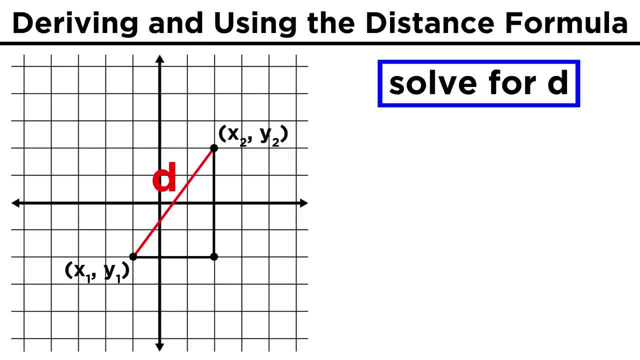 Now let's label the hypotenuse as D, The distance we want to know The legs can be expressed as the difference between the respective points that mark their ends. This horizontal line segment has a length of X two minus X one, since it only moves. 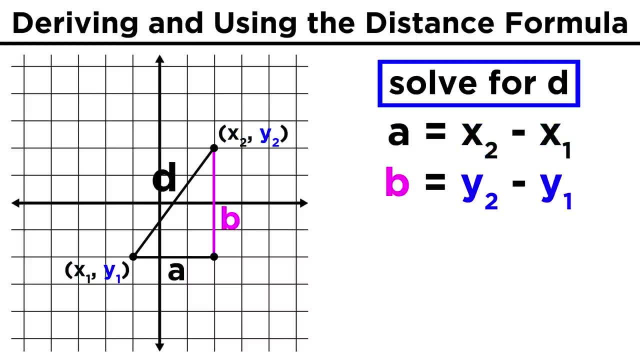 in the X direction, The vertical line segment has a length of Y two minus Y one, since it only moves in the Y direction. Now we just use the Pythagorean theorem: The square of this leg plus the square of the other leg equals the length of the horizontal. 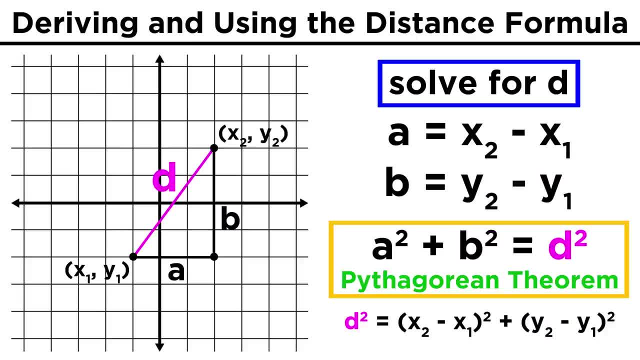 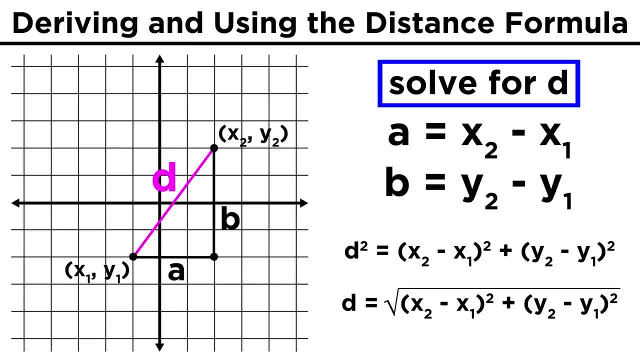 line equals the hypotenuse squared or D squared, Then all we do is take the square root of both sides to solve for D. We will only take the positive value here, as negative length doesn't make any sense. And there you have it: we have derived the distance formula. 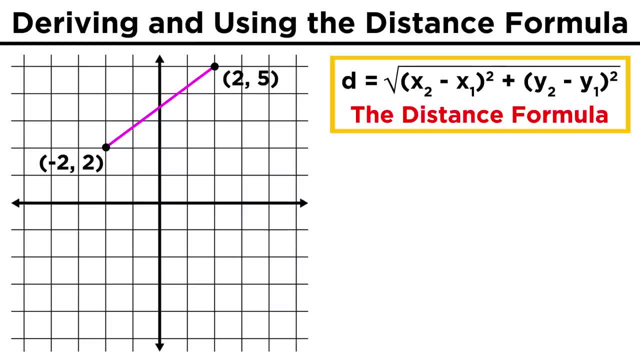 Let's give it a shot. Take the points negative two, two and two five. What is the distance covered by the line segment that connects these two points? Well, let's take our X- two, Take our X values and our Y values and plug them into the formula.